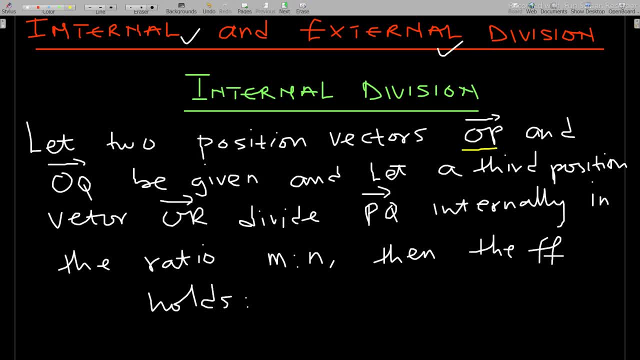 like i have here. okay, op and oqb given, and let's a third position vector, which is the or divide pq, the line segment pq. okay, this is very important internally, in the ratio m is to n. this is also very internal, like for sorry, it is also very important, you see. 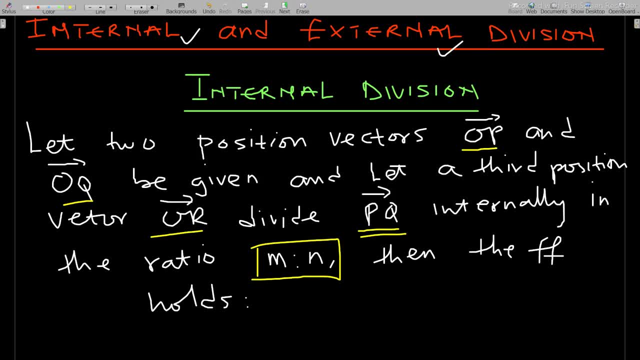 the line segment that this third point is dividing through is pq. this is very important. the direction of the arrows are very, very important. it can be qp that one would. that would be a different case, okay. so you know, dealing with vectors, your directions should be very, very important. 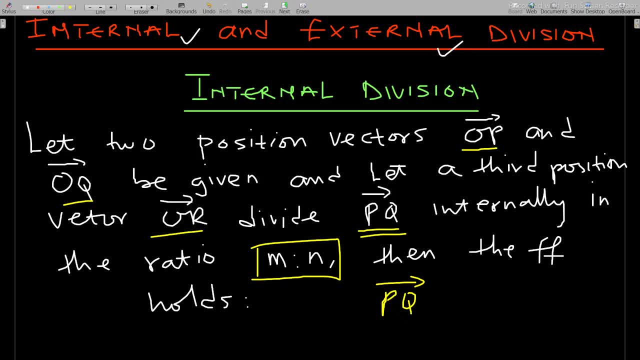 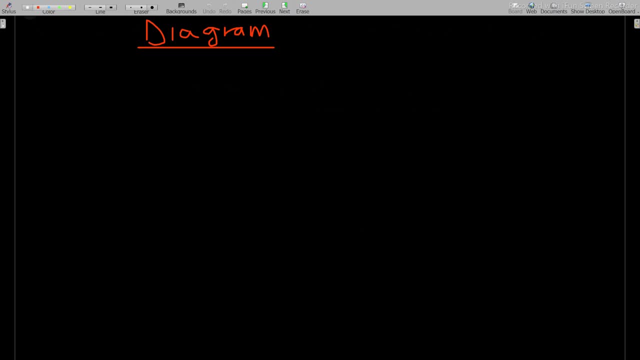 okay, then the following: so we are going to discuss about something that, if these scenarios are what we discuss, and then what i'm coming to explain here, or the diagram you are coming to draw here, really holds okay. so let's look at the diagram and see. okay, so we're saying that position vectors are. 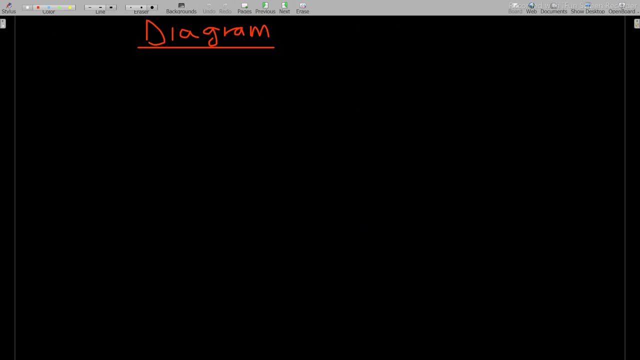 op and ok. and then the other vector is also- or, i mean they are all starting from a common point. okay, so let me say this is the- um. sorry, this is how the diagram should look like. okay, um, let me, let me have this okay. and let's say: this is the third side. i don't know. 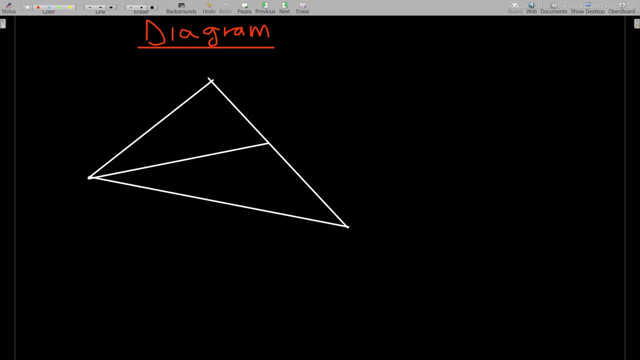 the magnitude of n and m. so let me put it in anywhere, okay, so that we just go ahead and do so. this is all, because they are all starting from oh. so let's see, oh is there, is this place and this, okay, this is op. and since we're giving op means this is how the directions are and or is also. 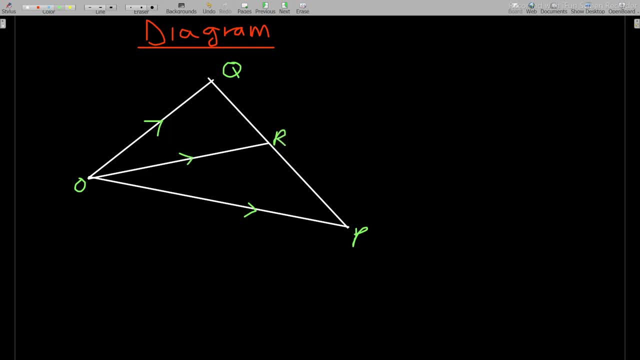 like this: and this is r, and we are saying that the point r is dividing pq, meaning the direction for the this side is this pq. this is how it's moving. it's like the direction is from q to p. okay, so this is how it moves. and then it's dividing it in the ratio. m is to n, okay, so m, the m will be for. 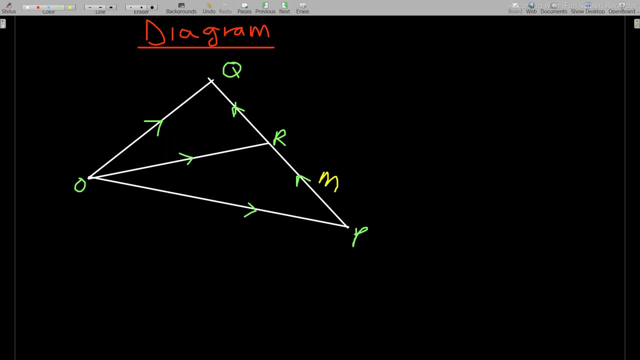 the p side, because it's if i dividing pq, okay, so from p, from p to q, like this, okay, so that is why you put the m that's at that part. okay, like this. so this is a scenario diagram for whatever that is happening there, and so from this diagram we can see a whole lot of things. okay, so from the 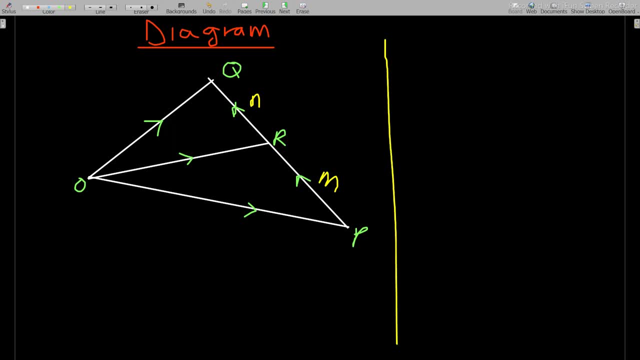 diagram. okay, so from the diagram. let's put it here somewhere. from the diagram or from the triangle, let's say triangle. anyhow, i want to put it okay from the diagram. okay, what can we see? all right, so the things you can see is that if you pick vector p, 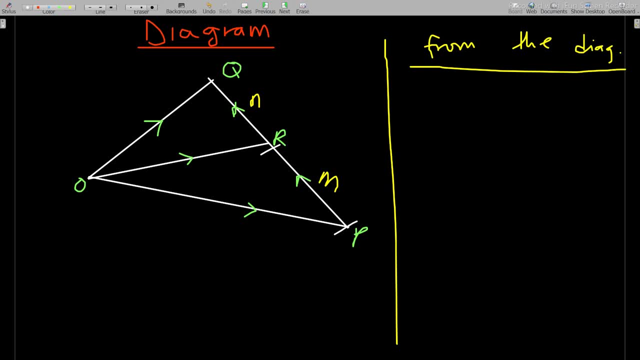 r, okay, meaning from just from this point to this point. okay, from p to r. so if you pick pr, like this, and divided by rq, let's say qr or rq, let's put it that way, because r is moving to q, so rq, like this, then you give us the fraction of the ratios. i hope you get it. so this is how the thing. 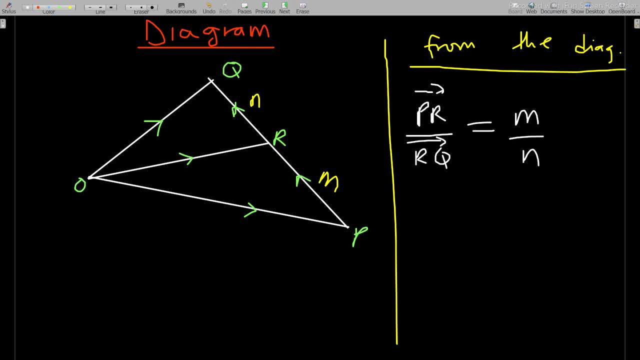 looks like. okay, now with this, let's go ahead and find pr and rq, okay, from our triangles- okay, we have a whole lot of triangles here, okay, so let's keep this somewhere. and then from triangle o, r, q, o is here, r is here and q is. 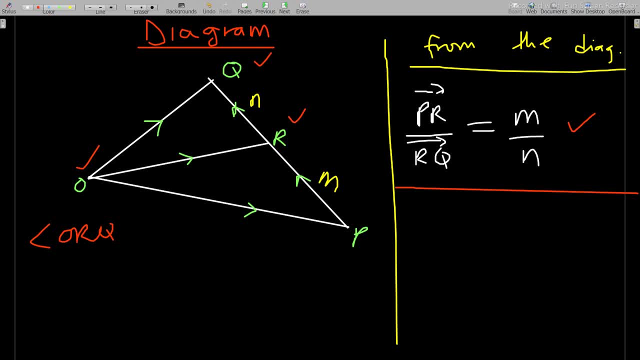 r is here and q is here, so i can draw that triangle. okay, i hope you can see. so let's try it to figure that triangle out and see how it looks like. okay, so the triangle is like this, this and this. okay, it's just this. okay, so i have my o here, my q here and my r is here, okay, okay, let me put it. 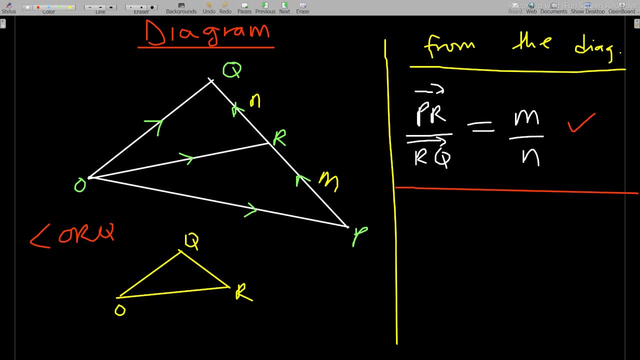 here. this is how the arrows look like. i have it here and i have this one here, i have this one also going that way. so, from this triangle, what can we say? we can say that, um, from the triangle of vector addition, the ones that are moving in the same direction, 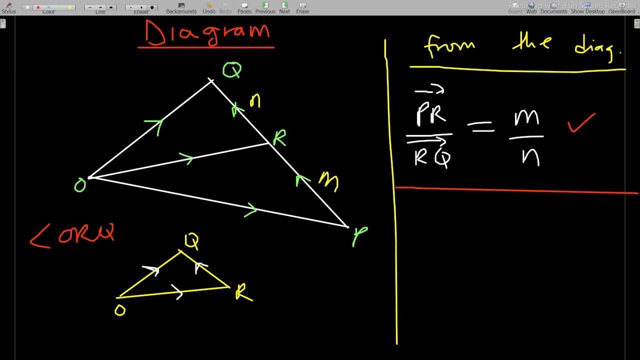 because you can see that o? r is moving here and rq is also continuing like that. okay, so the assumption we go together to the one that is moving the counter direction: okay, that's what we just discussed in our addition of vectors in the triangle law of vector addition. so, or, okay, plus rq should be equal to oq. okay, and 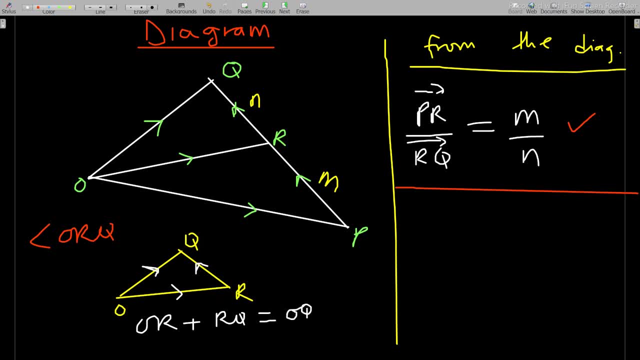 from. you know position vectors. we can name the rq and then oq and the rest you can see. oq is small q, okay. op, small p, let me put them there. and or is more r, okay. so it means that this rq here i want to make, there is an rq in this, okay. so i want to make rq the subject in this one, so you can see. 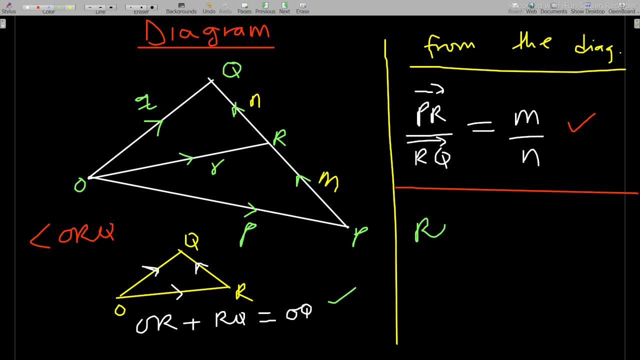 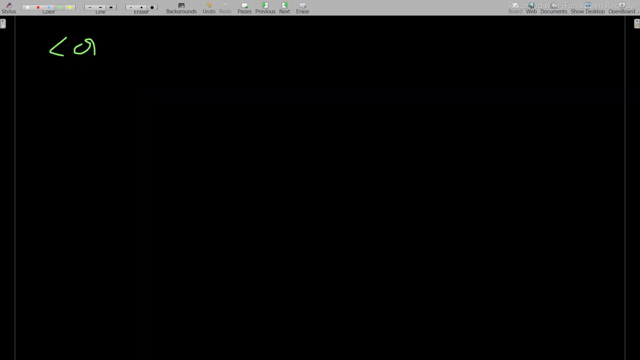 that rq in what i've just written here is equal to oq minus or okay, and this is the same as small q minus small r. okay, so we keep this and go ahead and find from triangle opr: okay, sorry, opr, okay. so let's go ahead and look at triangle opr. this is triangle opr, this is o, this is p and. 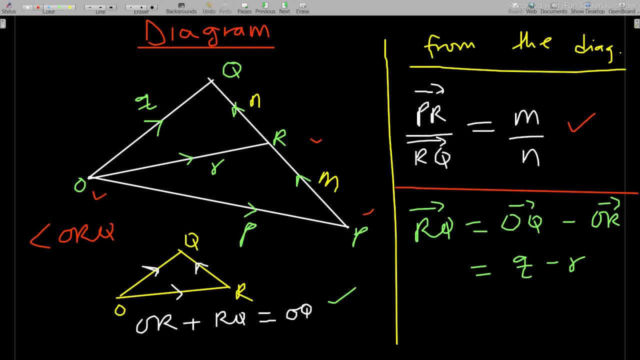 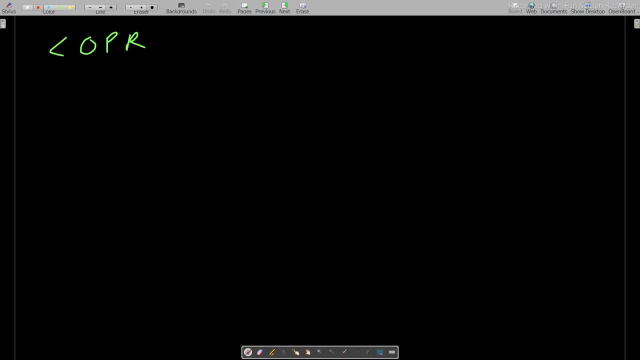 this r? okay, so i can draw that triangle as well. okay, so we can take a pen and pencil and draw that triangle and see, that triangle looks like this. okay, let me, let me draw it for you. oh, let me. okay, it looks like this. let's, let's draw it like this. okay, so that is it o pr. okay, so. 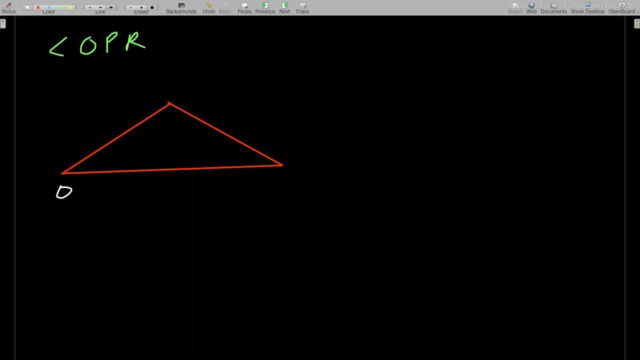 o is here, p is here and r is here, and this is how the directions are. okay, and it's this one is moving to that direction. with that one, two, we can say that op plus pr- okay, it's equal to, or. i hope you can see this. 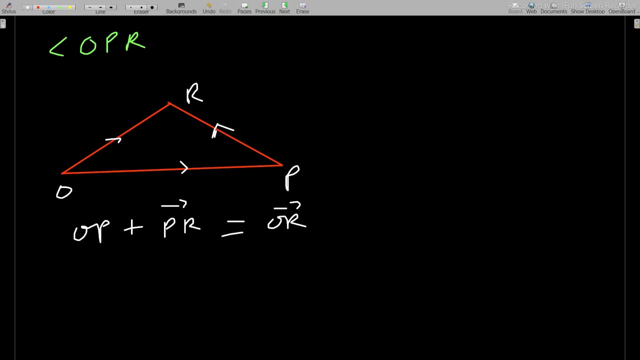 now we know that pr is also equal to or minus op, which is the same as small r minus small p. okay, so go ahead and with the equation that we wrote you, we said that, let me write it here back. we said pr, okay, over our Q, should be the ratio or the fraction M over N. and now you know. 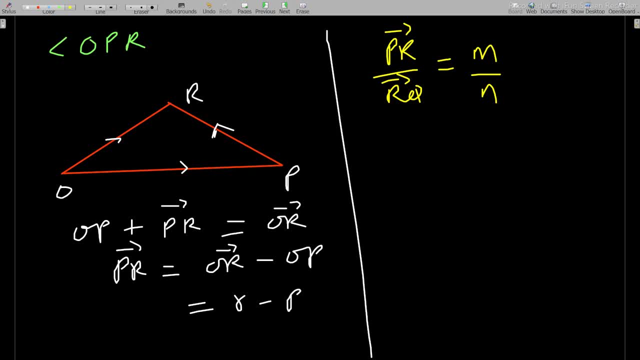 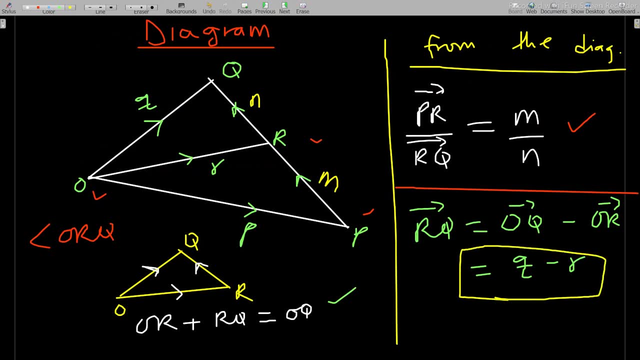 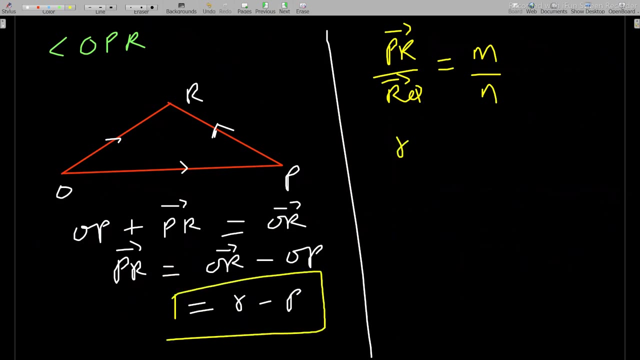 PR. you know our Q. okay, if you remember this, our Q, our Q, is Q minus R, this one, and our PR is also this: okay, so you put them in the, in the this, this equation there, and then this is what you get. we get PR is what R small R minus small P. 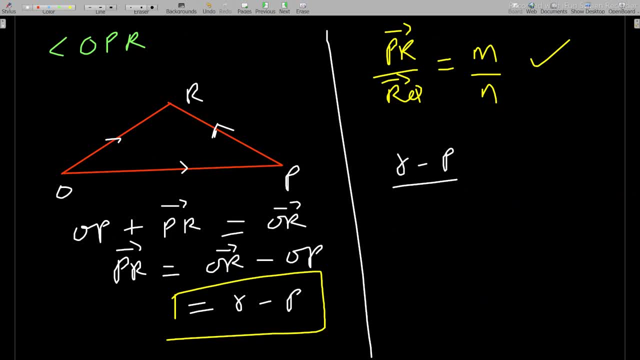 over this QR, and that is small Q minus small R, and it's equal to M over N. okay, so, simply, what want to do is want to find the third position vector that divides this. okay, so you want to find this, the formula for this, because always OQ and OP will be connected. 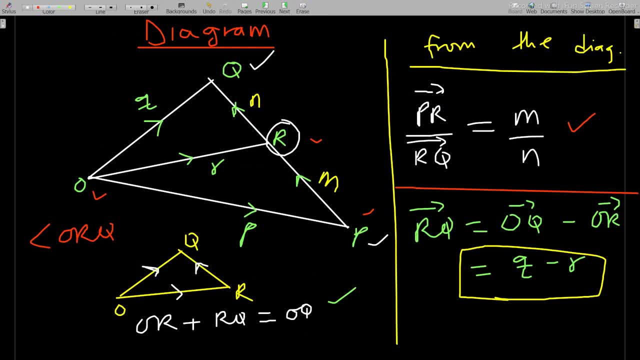 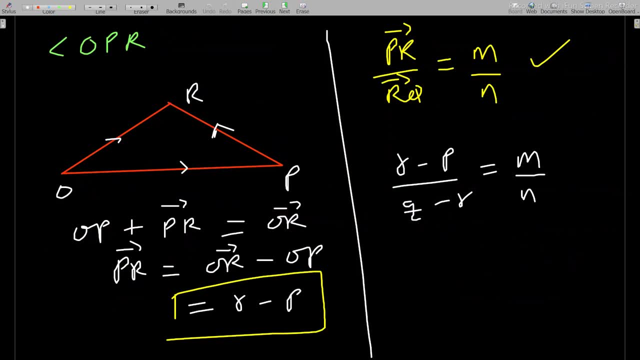 so we pair things right giving. so what I want to do is want to find a or. okay, so the or will give us the small R, obviously. so it means that I have my n into bracket. R minus P is equal to M. into Q minus R. okay, so with this nr minus NP, we go to M, Q, okay, minus. 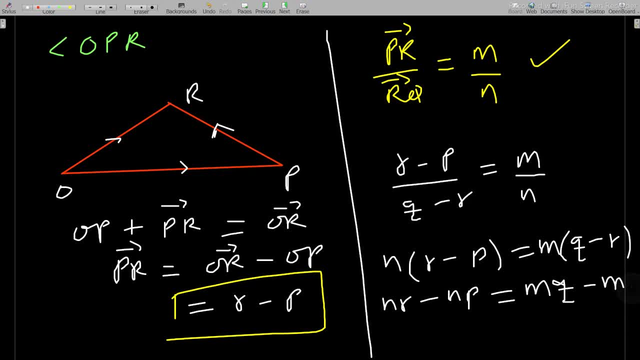 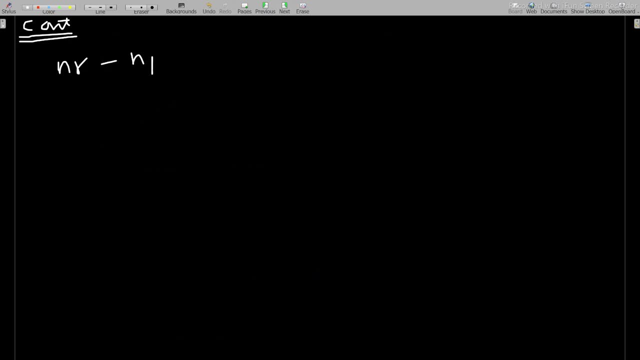 mr. now with this one you can make. you want to make our subjects so quickly. let me write it here. you have an R minus NP is equal to M Q. okay, minus, mr. so you put all the arrow at one place like this. so you go to M Q plus NP. 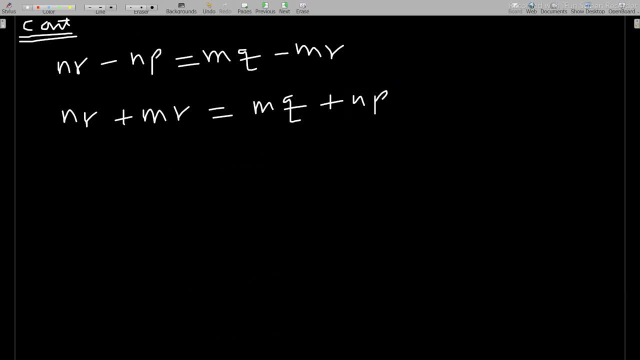 you have my R out, M plus n, or you can say n plus M, anyhow you want to see this- plus NP. this means that R will be equal to M, Q plus NP, all over M plus n. so the position vector for a point, that device, the line segment, P, Q. so look at, look at. 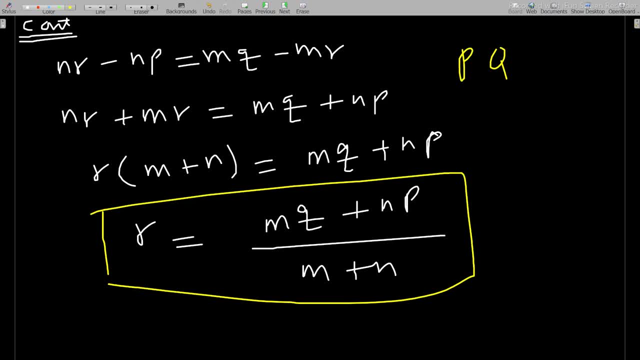 how the sediment is like pq. okay, so it's from p to q. then it means, and it divides in the ratio, m is to n. so always you take the first ratio, multiply it to the small, the last one, that is the kill. okay, so it's like: 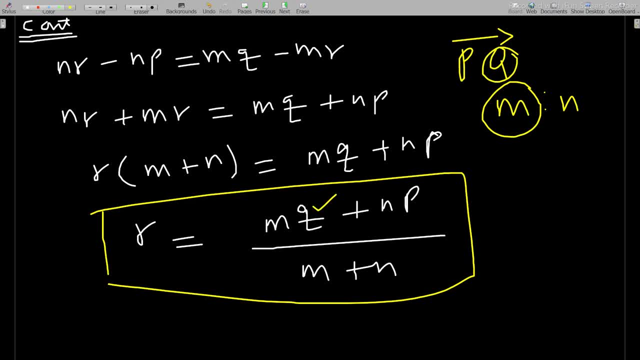 this. then, plus this last ratio, multiply the first vector, which is the p, over the summation of the ratios. okay, i hope you get it, so always check your directions very, very well. okay, we can say that, find the position vector, or the point that divides the lines that you might kill r. 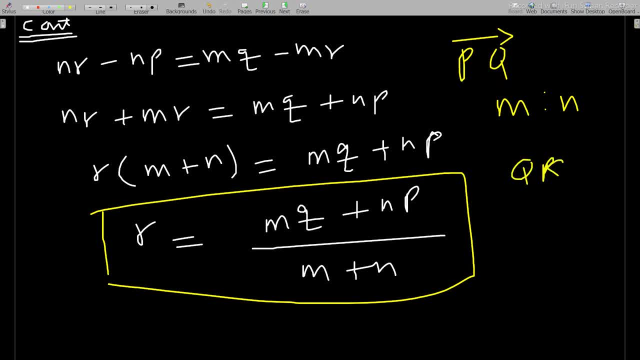 or it's a qp, so it means qp. if it was qp, this would have been different. i hope you get this. so just look at how you or your vector or your question is being given and you know how to go about it. so this is the. this is the formula for the internal division. let's quickly go through. 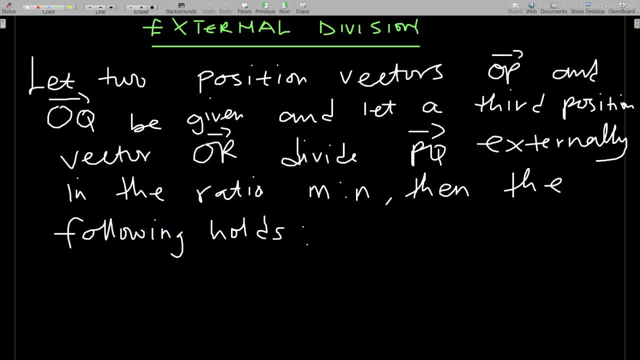 the external division and we'll be done for this video. in the next video we'll take examples. okay, let's do position vectors op and oq be given. that is op and oq. and let's a third position vector or divide the line pq. so is this one to: is pq from p to q externally in the ratio? this, okay then. 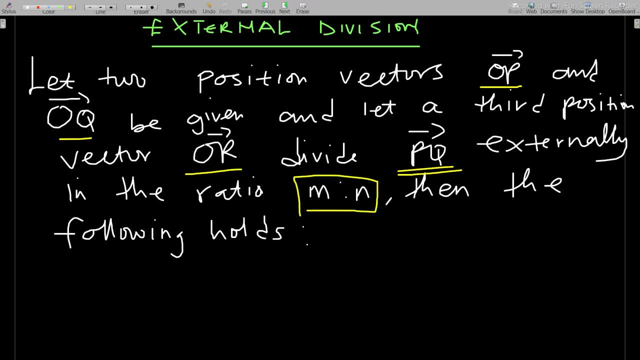 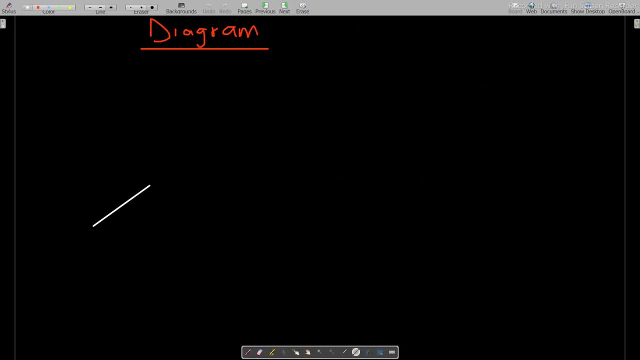 the following: host that one to go through the diagram and after the diagram. you understand, okay. so let's say: i have my point, this okay, let me put it here like this: okay. okay, let me let me put it here: all right, this is, this is very okay. so it's like this: 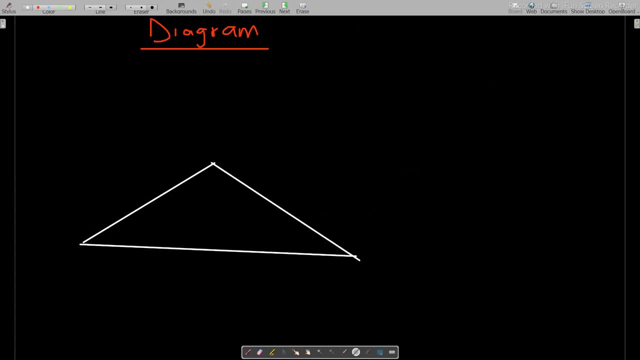 um, yeah, this is okay. so there's an external other point that divides this in a ratio. so it means that point should be an external point, shouldn't be part of this. so it means that point is from somewhere here. let me put it here, okay, so it's, in short, dashes like this: this is how the diagram looks like. okay. 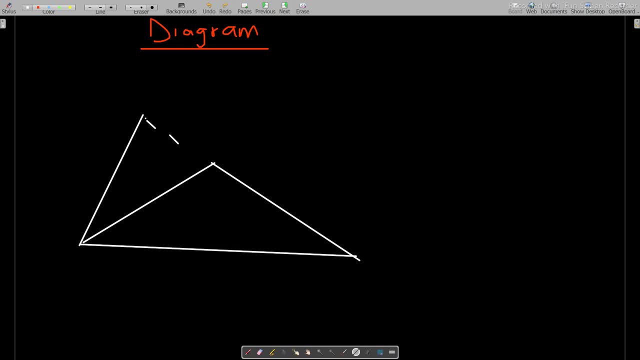 this is how the diagram looks like. okay, it's a standard division. okay, so it's like an external part of it. okay, so with this one we have, we have- um, uh, ought to be here as usual, our peace here and our cale is here this time. that is why i'm saying that there is understand. 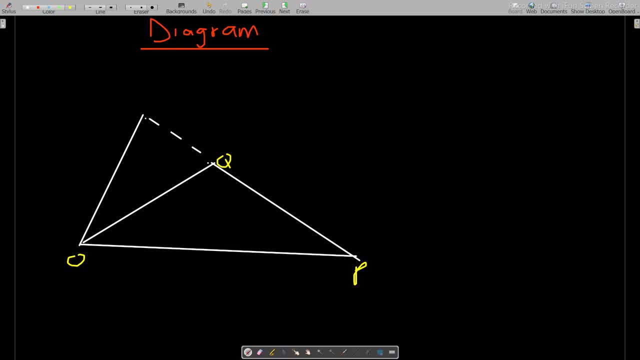 an extension of our diagram. now, r is right at this side, okay, but it's dividing the lines, segment pq in the ratio. m is to n, meaning from p to r is always what our m, that is what our first, our first, said. so, from here to here is actually our m, and from this distance to this distance, it's actually our m. 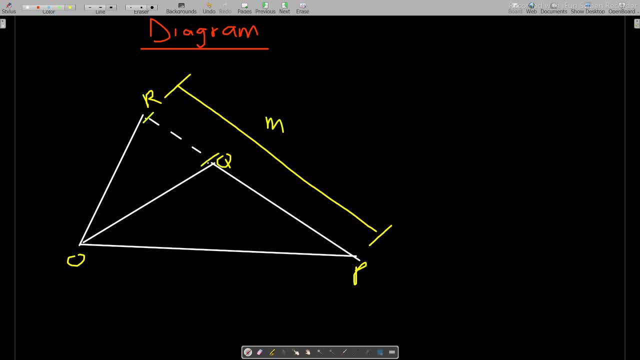 to the distance is actually our n. okay, so with the external division, this is how the diagrams look like. okay, now op. is this ok, is that, or is that? so pq goes this way, so it means pr also go in the same direction. okay, so this is a scenario. then everything becomes as simple as that. okay, 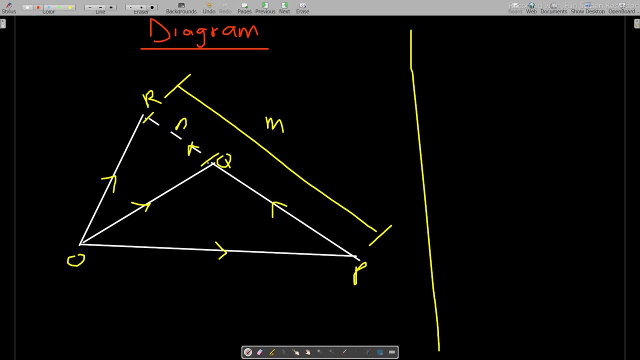 if this one true, you can see that if you take the vector p, r and divide it by vector, let's say qr, okay, the same thing will happen here. we'll get m over n, okay. so we just go through some of the triangles and, like refers, that we just 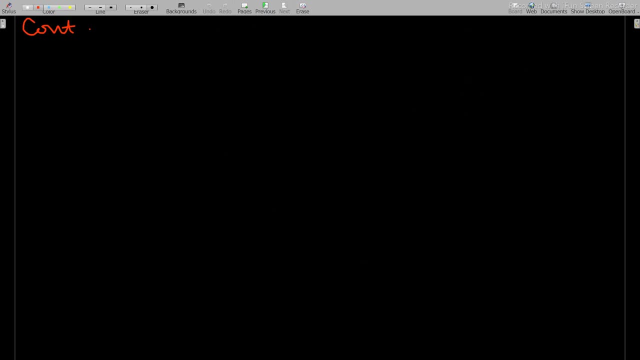 you know, do what we can do and then get some formulas out. okay, so from triangle o p? r, so we can go back and check o p? r. okay, so let me go and draw that one for you. okay, opr looks like this. let me pick my pencil and draw it. 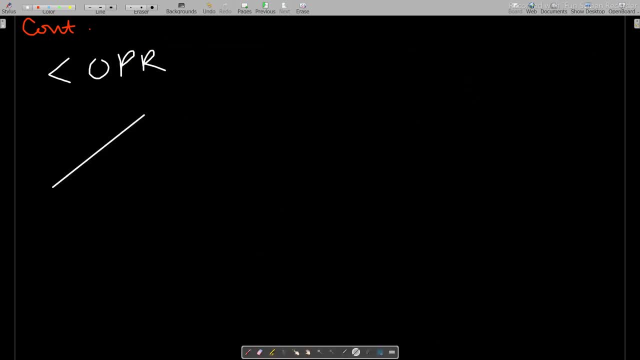 this is how opr looks like: o- p, sorry, pr. okay, and this is small p, if you remember, and this is small r. okay, so this is how the direction goes. you say that you're moving from p to r, so it means that from this triangle we can say: op plus pr is equal to, or okay. 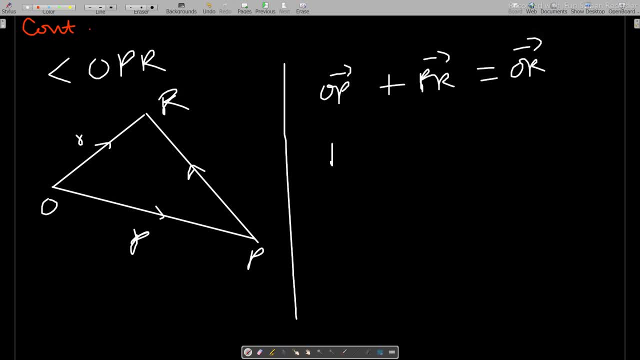 meaning pr here is simply- actually- we have done this in our first discussion- that pr is always equal to the position vector of r- small r- minus this position vector of p, which is the small p. i've done this before. that is the line joining two points. okay. 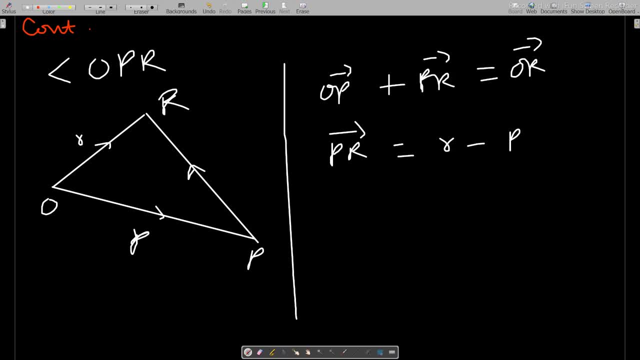 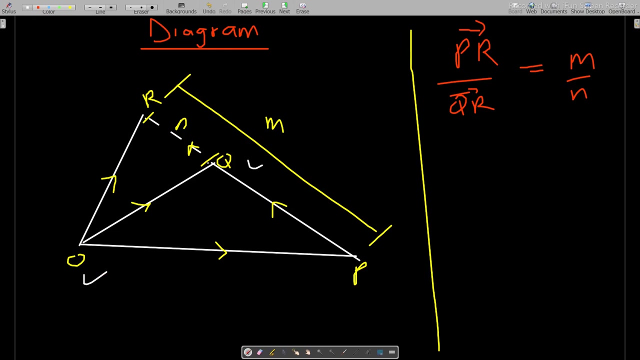 all right, so this is pr. then we go ahead and find for triangle um, o q r. okay, o q r that one to go through it and see: now let's go ahead and check triangle oqr. oqr is from here, o q and r like this: okay, that is how it looks like and the diagram looks like this. 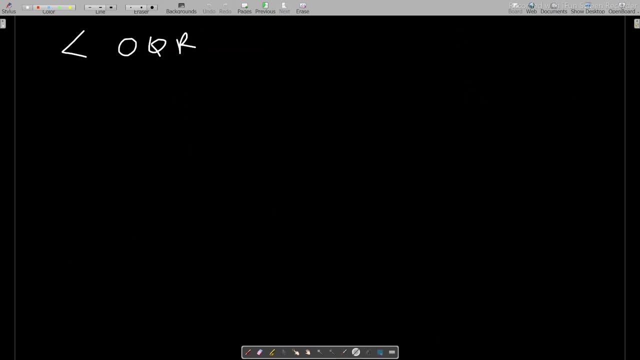 from here it looks like this: um, this one, let me draw it as it is in the diagram. okay, okay, all right. so this is how it looks like and with that, that one, two, you have oh killed, and r is here, and this is how the directions look like. okay, this is my r, this is my small q, so it means: 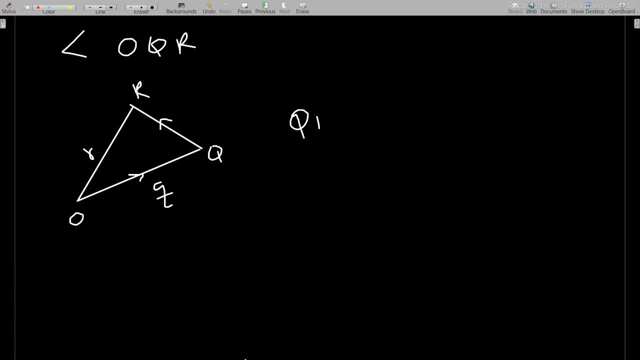 qr here. i'm just writing it straight away, i know you can go through it: oh q plus oh p, qr is equal to r. so, simply, qr will be equal to small r minus small q. okay, so this is it for my qr from this triangle. now, with this, let's go ahead and write a formula. we said that pr over qr is equal to m. 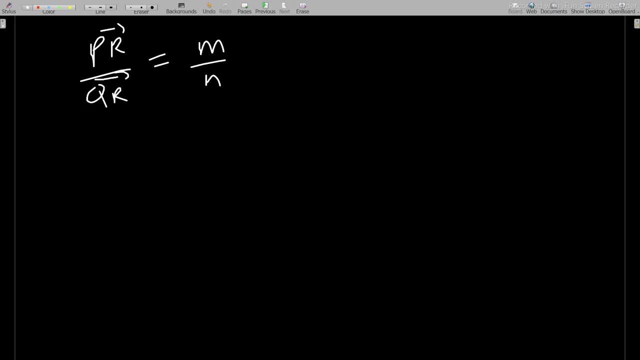 over n. so with this one pr was given as what? go ahead and pick it this pr. it is r minus p and qr was given as r minus q. okay, so we go ahead and bring it inside our formula. so r minus p. this is it okay? over r minus q. small q should be this: over n: okay. 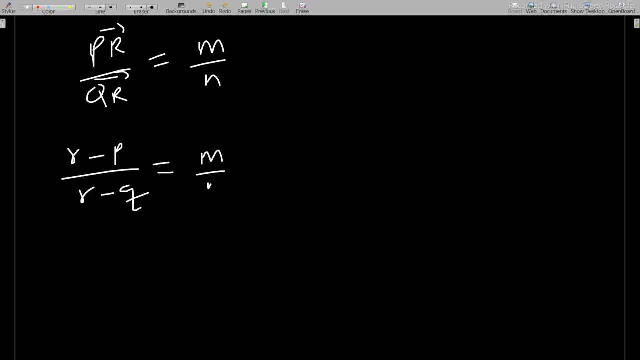 now i have my n into r minus p is equal to m into r minus q, so i can make r a subject here. okay, r minus n p should be equal to m r minus m q. okay, now this: we can say that n r minus m r should be. 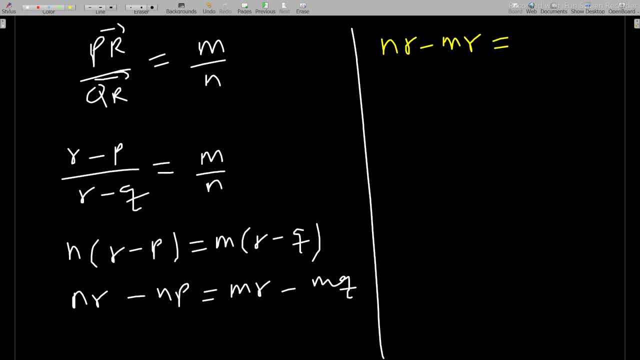 equal to n p minus m q. okay, so i have my r out. n minus m should be equal to n p minus m q. so it means i have r equals n p okay minus m q over n minus m. this is correct. okay, this is very correct for external division. now other books. we want to simplify this expression in a different 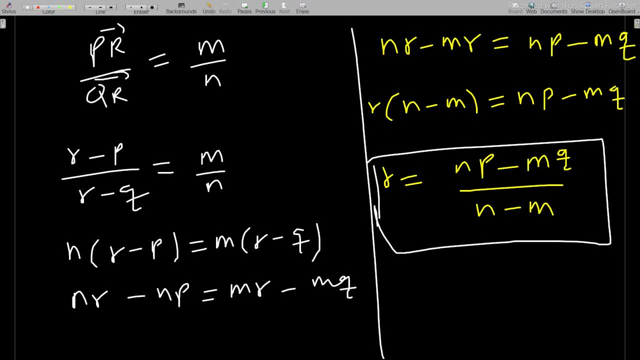 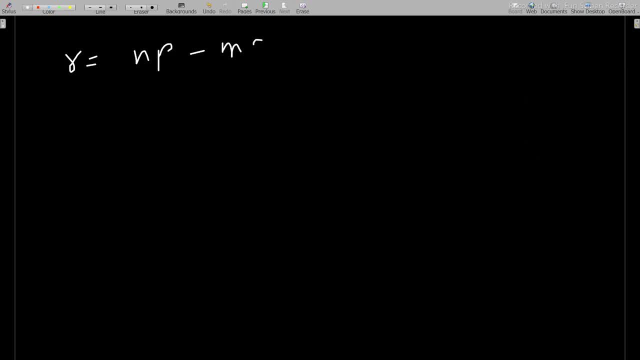 way. okay. so having r to be r is equal to n p in the external division over n minus m. okay, other books: we want to continue this and say that if i factor negative one out in the third in the numerator, i'll get m q minus n p. okay, now, if i factor negative one,